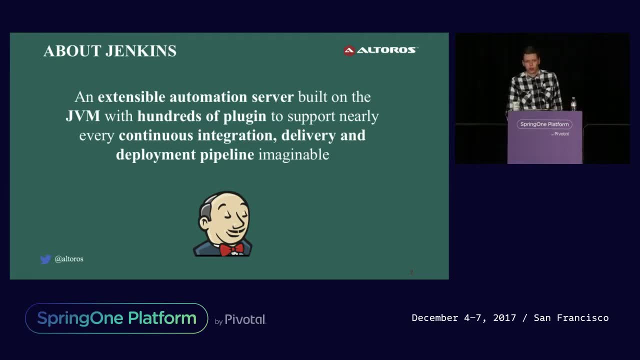 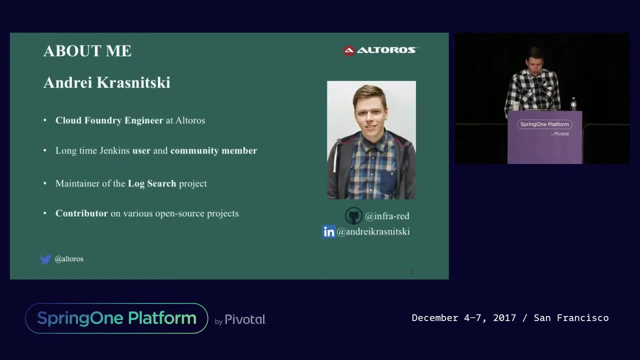 is not my main CICD tool. I work with like many CICD tools like concourse, GitLab CI, Travis, CI- but still this is the tool which we are using the mostly, And we all should agree that Jenkins is a leading CICD server at the current moment. My name is Andrey Krasnitsky. 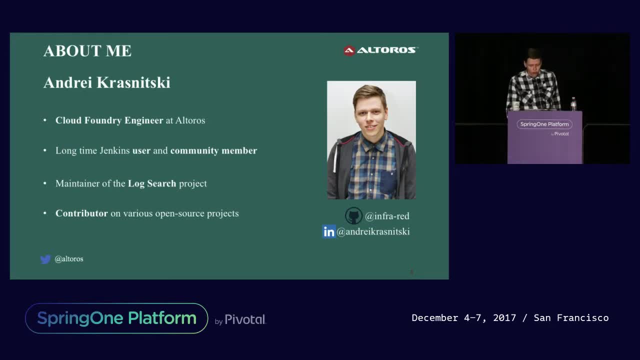 I live and work in Music Bell. I am a software engineer at Altorus But since we are working mostly with the Cloud Foundry, we like to call it Cloud Foundry Engineer. I have been working with the Cloud Foundry and Jenkins from the beginning of my career And this was tools which I began. 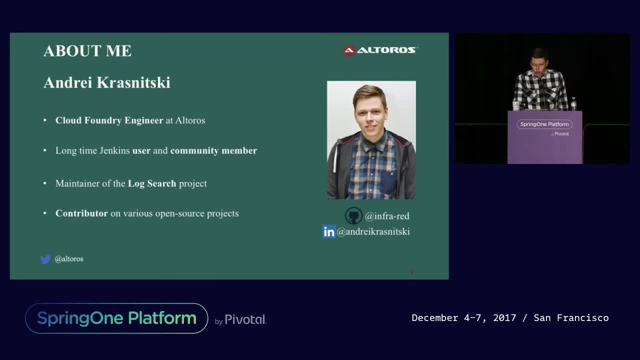 to study at the very beginning of my software journey. I am also maintainer of the project. If some of you are already working with the open source version of the Cloud Foundry or with the PC version of the Cloud Foundry, I have been working with Jenkins from the 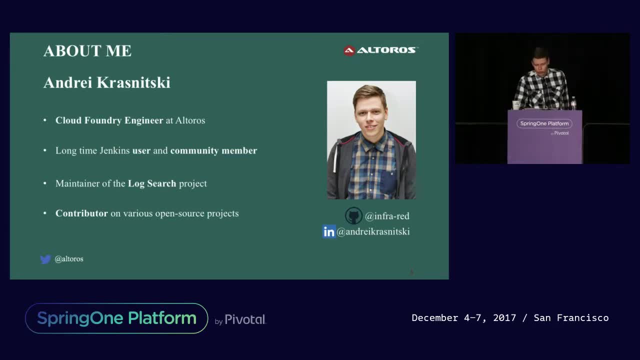 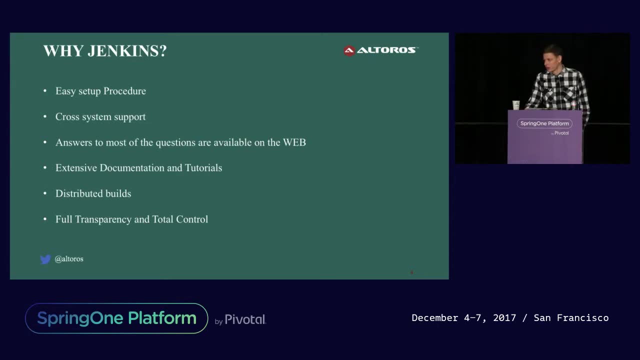 beginning of my career. I have been working with Jenkins from the beginning of my career, ECF installations. you should know something about this project. So the main question with people asking why we're still using the Jenkins because here are too many CI service which already solved all the problems. 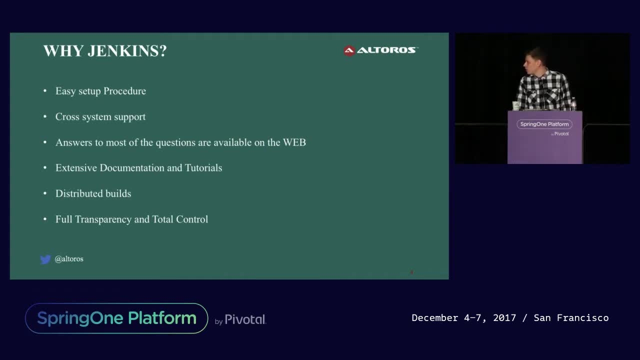 which was the Jenkins. but I have some simple reason for it. The first of all, Jenkins is really easy to set up because you just need to download the Jenkins certified, run it with the single common Java jar in any virtual machine on your favorite cloud provider and that's all. 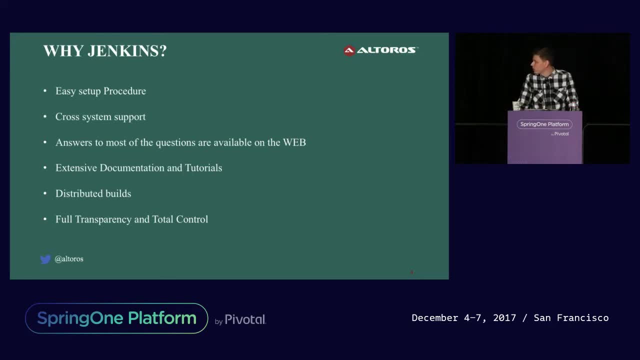 And if we are talking about the PCF tile, which I'm here representing, you just need to download the style from the pivotal network, import to the PCF Ops Manager, click Apply Changes and that's all You will have like fully working Jenkins environment within your 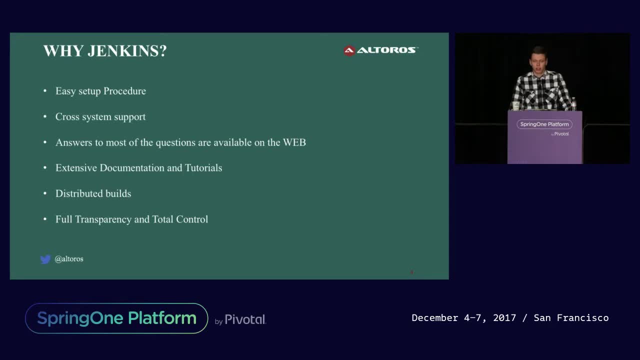 beautiful Cloud Foundry infrastructure. So Jenkins has a very low input threshold because when you're starting to work in, you can go to the web UI and you will see that all buttons, all text fields, all the checkboxes will be provided with description. 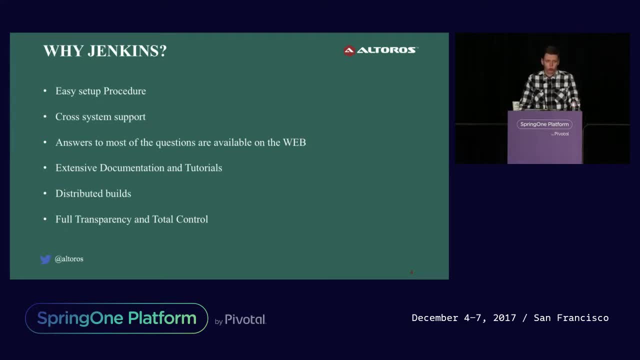 on what should be included there. Jenkins support all of the environments. You can run your Jenkins master and Jenkins build slaves on any environment. You can run the half of the Linux, half of the Windows environment And Jenkins has a really great documentation. 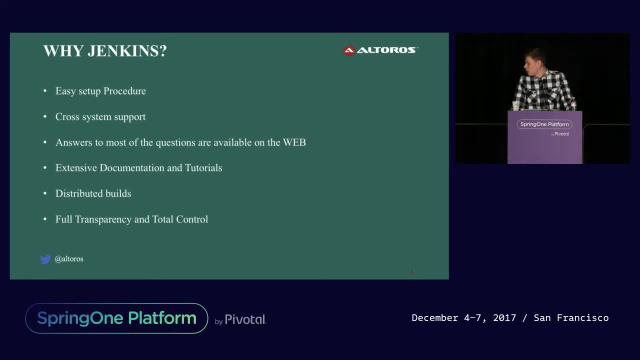 Even Jenkins plugins has a great documentation, So you almost may be sure when you're trying to solve some problem, that this problem was solved by someone over the Internet. And finally, Jenkins is easy to customize. You can create your own plugin if you have like basic experience in Java and install. 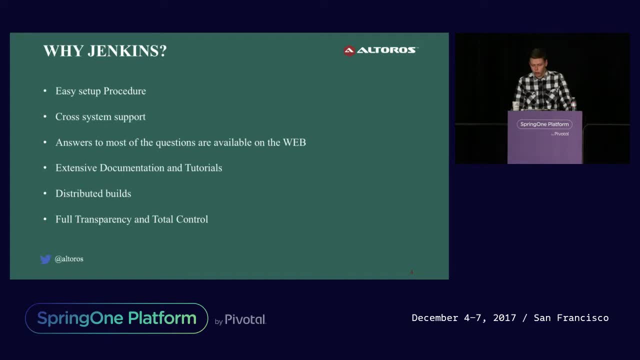 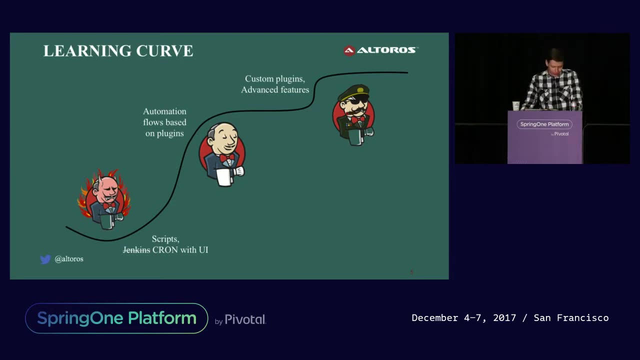 this plugin in a couple of comments or in a couple of clicks when using the Jenkins web UI. So sooner, or usually later, we will start into implementing the CI-CD processes on our projects. Usually we like to begin with the basic bash scripts. 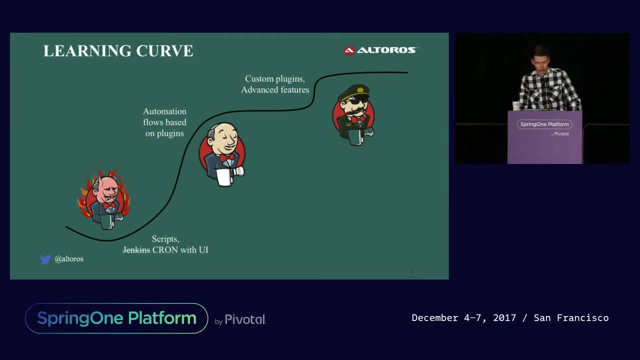 And usually the most of people actually stopped on this step. But if you will continue to improve your CI-CD process, you may achieve the many benefits from it, And in this speech I want to focus on some of the features which will be will was included. 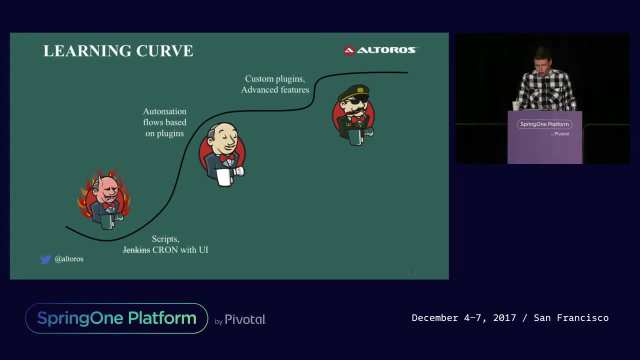 in the Jenkins, but still people ignore them, And I will show some tips on how you can, How you can save lots of time, even for the entry organization, when you're using the features which comes from the Jenkins out of the box. So it's usually all about the pipelines. 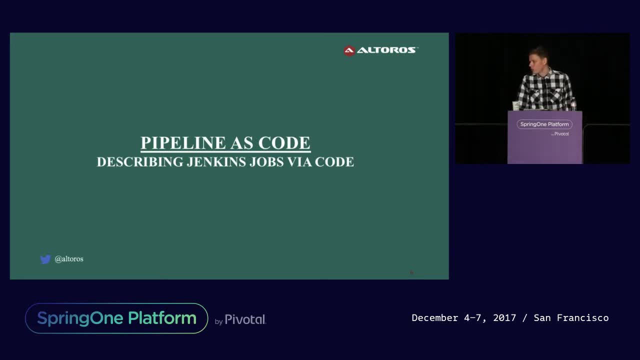 So when you start the continuous integration journey, you need to understand that this process is more complicated than just our usual build, test and deploy steps. Each of these elements should consist of many other steps, And these steps usually are interdependent. Why this algorithm should look like following: 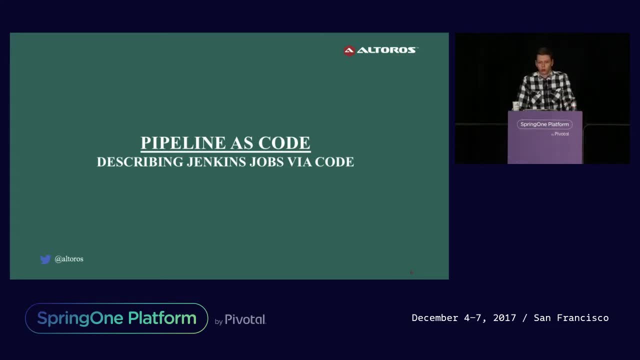 For example, you can run some unit tests. Then you need to build your application, You need to create like services which will be required by your application in the cloud, and so on. Also, you should always remember to include some additional logic to rollback service. 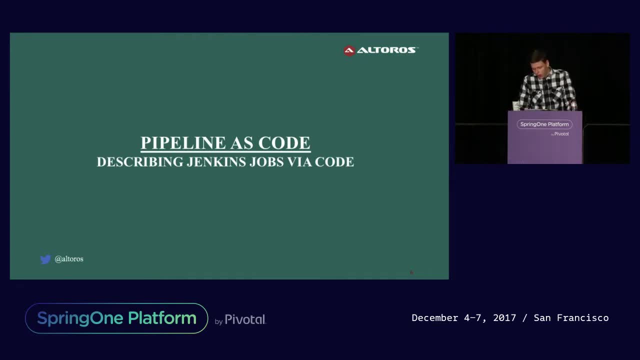 if some of your position is not working Absolutely. deployment tests were failed and I would like to focus on the some tools which will help you to build the powerful pipelines with the Jenkins. so how exactly can Jenkins pipeline help you to improve your CI CD process the most? 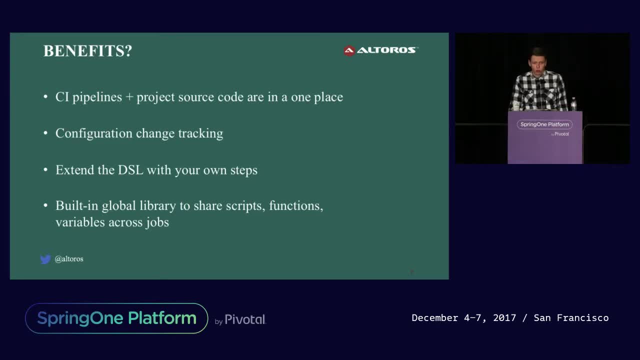 obvious and that your pipeline code will be stored in the your git repo or any version control system that you're trying to use, and in case of any disaster, you will easy to recover from there. you will, you can easily recover from this Jenkins file in the pipeline and since you're storing all pipeline, 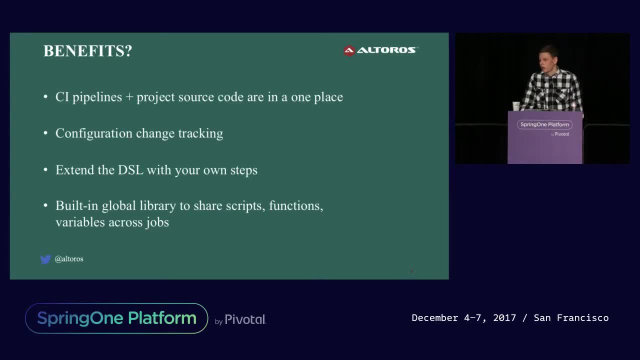 configuration in the version control system, you can easy check what was changed, when these changes were made it and who exactly made this change. also, one important feature that Jenkins pipeline provides is that you can- you can implement your own features inside your Jenkins file, and all this feature will. 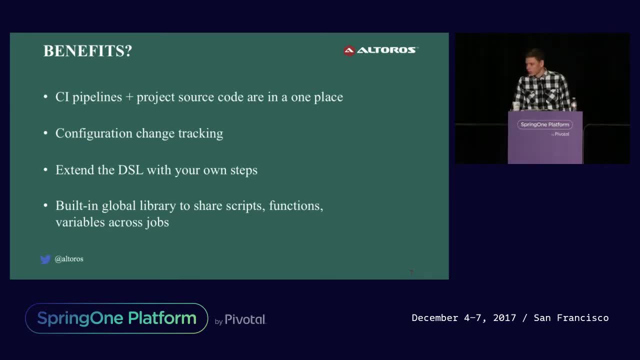 be available for all of your user on the Jenkins serve, for example. if you know that you need some difficult step, but you need, you know that one person from there- your team- already solved this problem. you just need to import this function and you cannot use this function in your own. 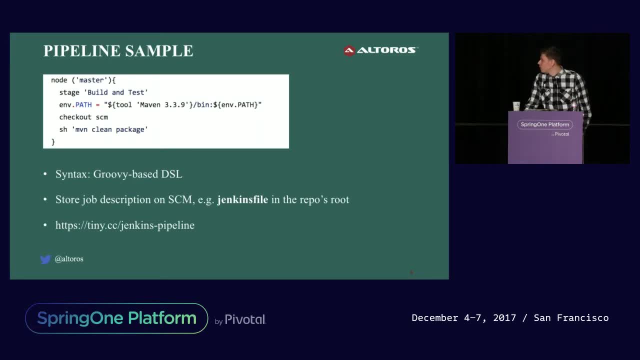 pipeline file. so here is a simple pipeline example. you can see that this is pipeline file is based on the groovy base DSL. some people may be scared because we all know that our modern CI system use the yaml pipeline yaml syntax, but it's not more complicated than default yaml which we are working in the. 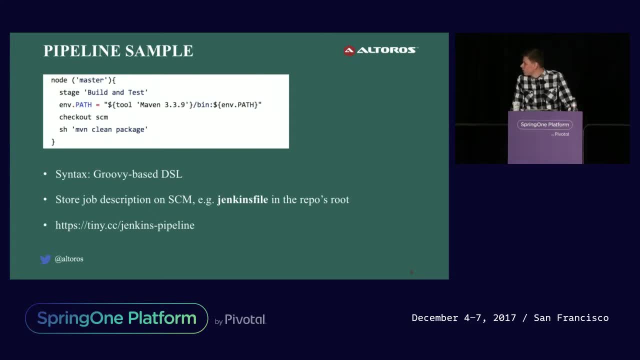 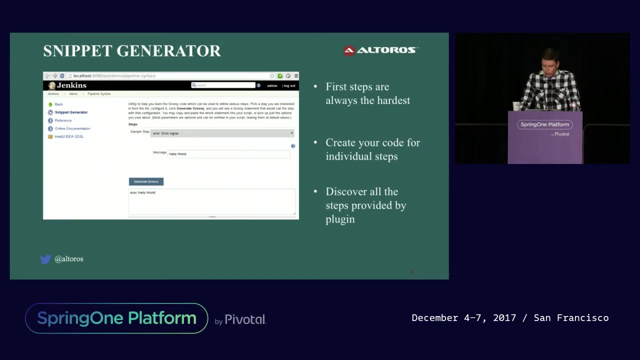 most tools and besides I added here the link it's provide like good tutorial which if you want to start working with the Jenkins pipelines. so Jenkins includes good feature which called the snippet generator. it can help you to begin working with the Jenkins pipelines. I usually use a tool to discover, like 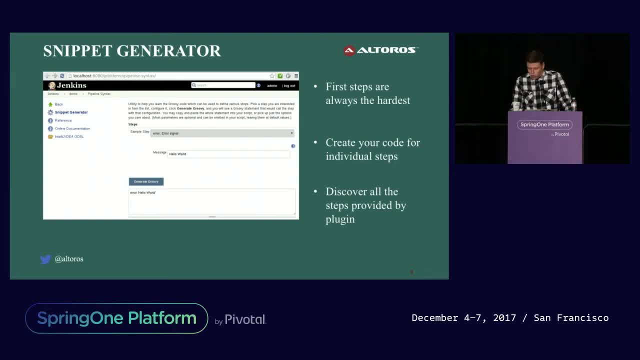 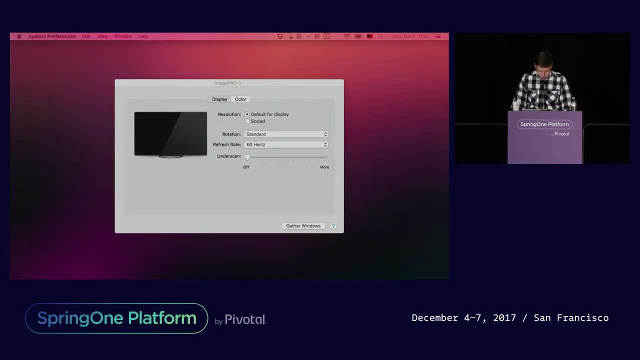 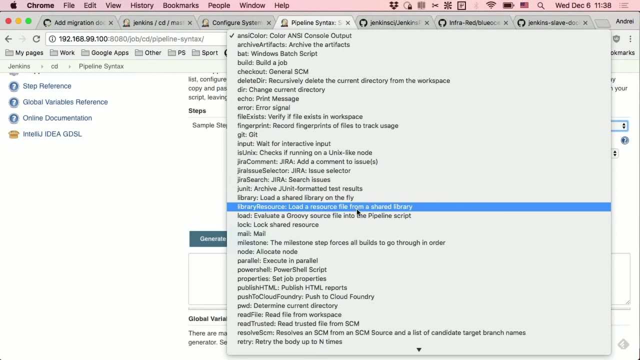 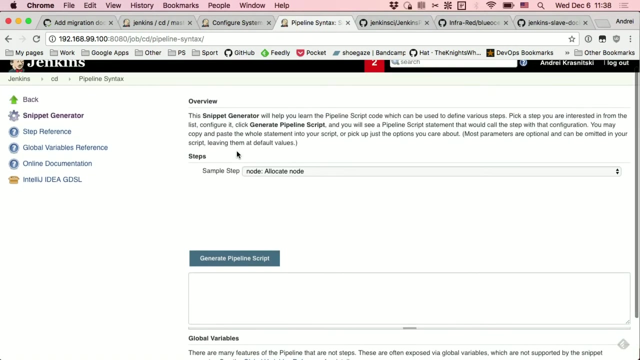 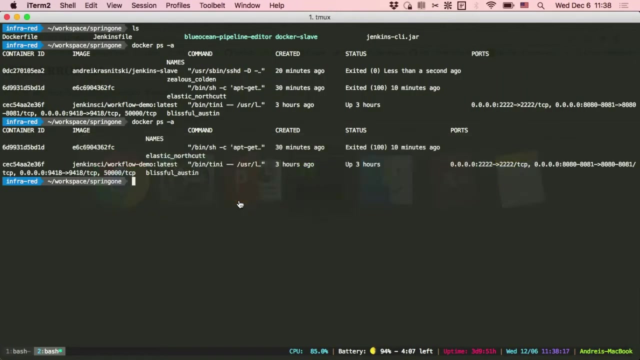 steps which provided by some plugins. so let me show you how it can use a source, our Jenkins lines, for example. we want to just second, for example, we want to create new Jenkins file which will be executed on the master note. so I will check the. take the note. okay, looks like we have a problem. 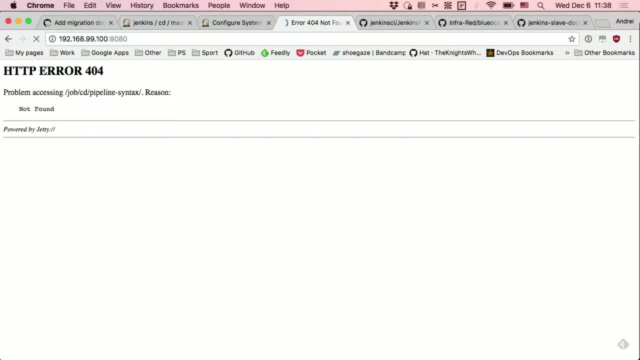 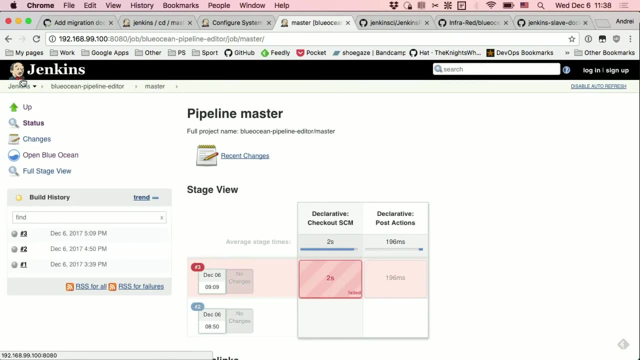 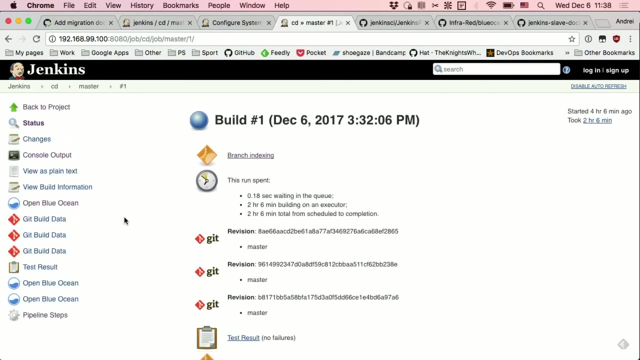 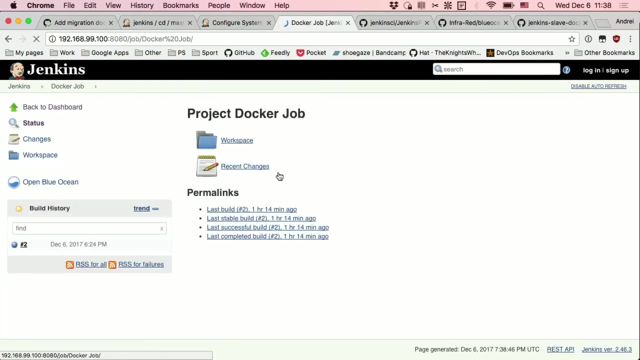 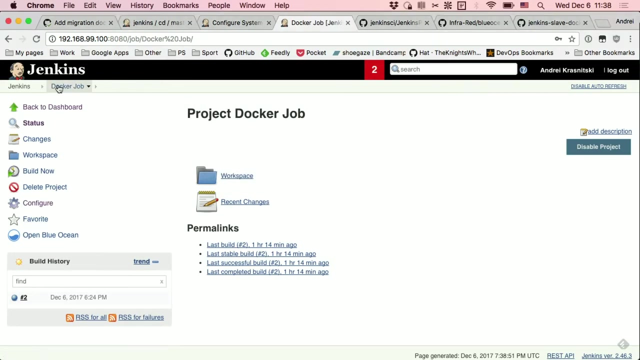 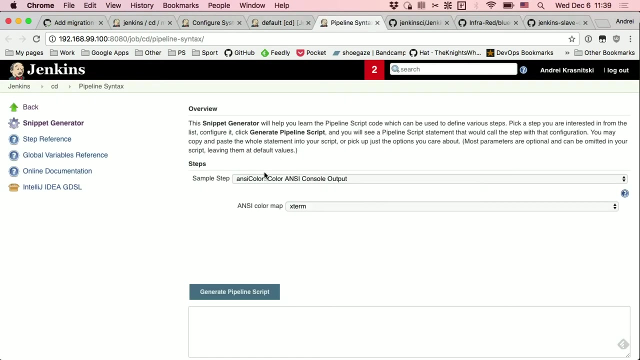 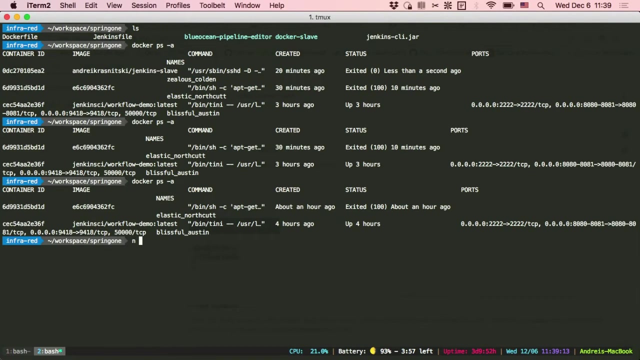 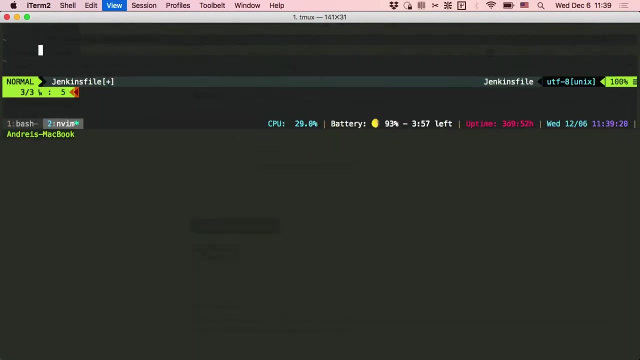 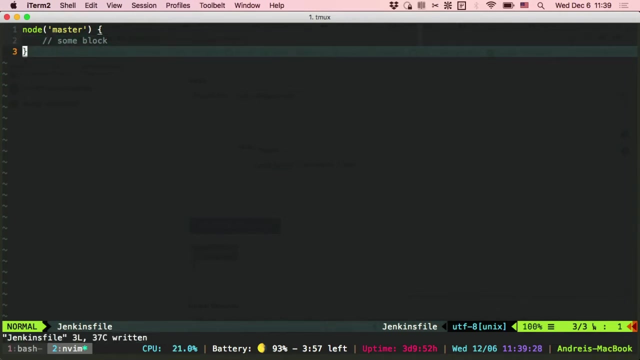 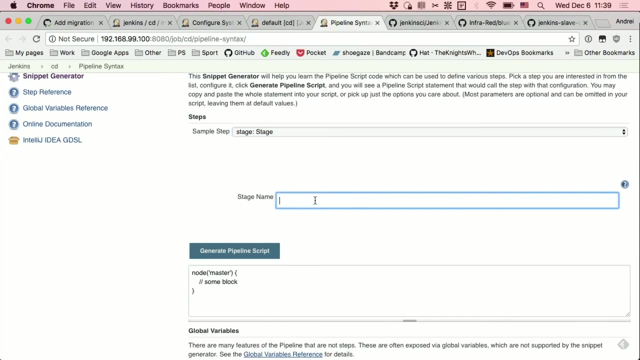 just a second. there we go. so we will like to run this pipeline on the master node, so we will have like simple pipeline snippet which we can use. so let me put it in the our Jenkins file: okay, so let's add some additional stage like, for example, we want to build and: 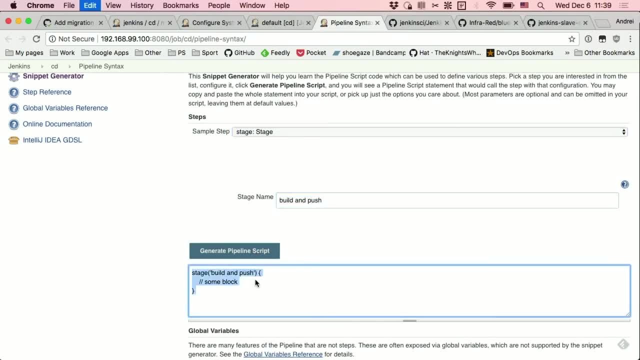 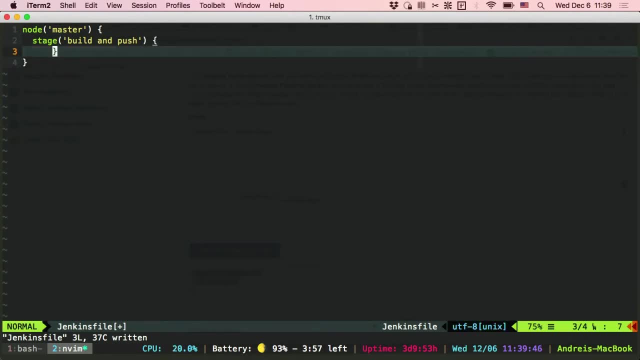 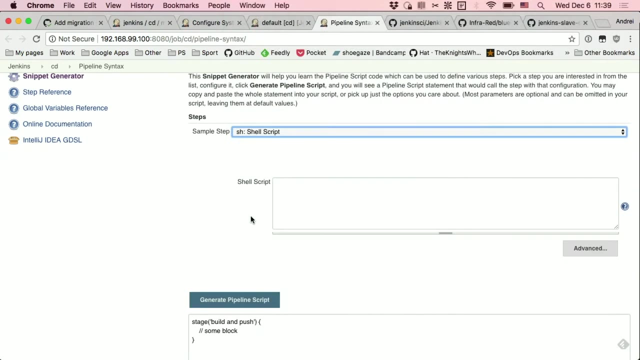 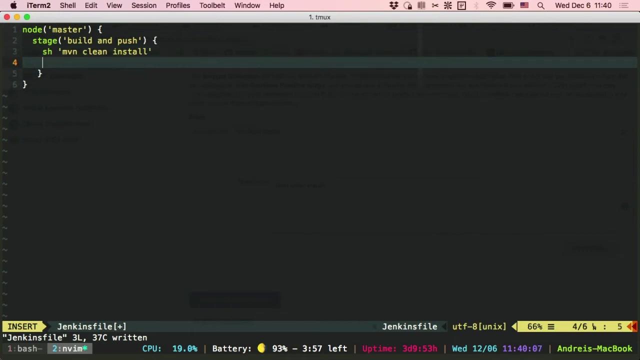 push to our Cloud Foundry so you can add stage here and, for example, the next. our steps will be to execute- I've been clean install to prepare our package. to push to the Cloud Foundry, we will use the shell script and after that we can add some additional tasks to push this. 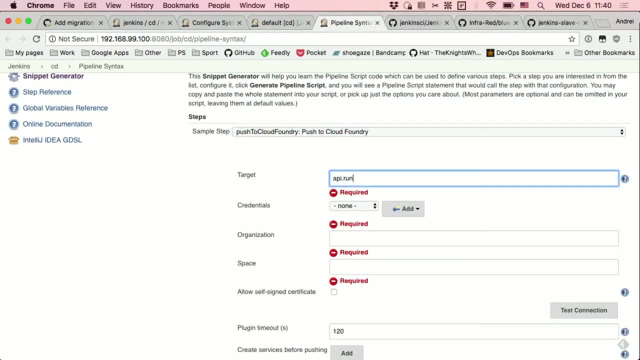 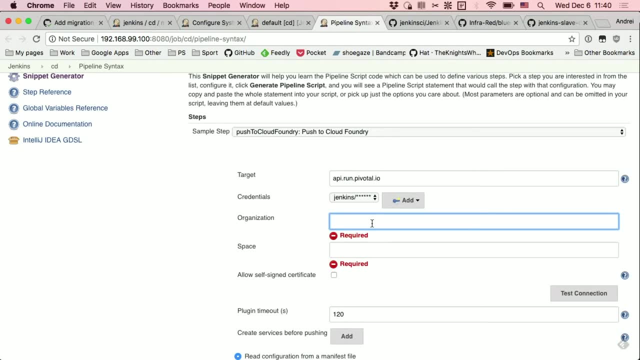 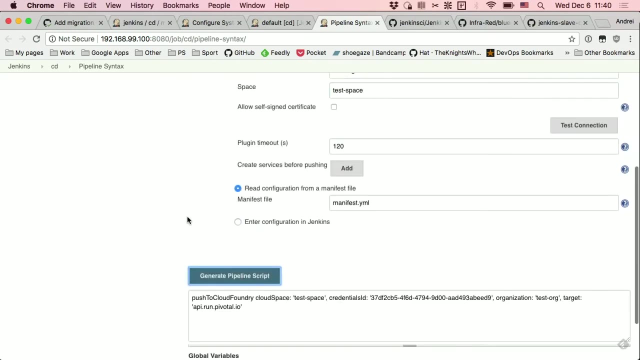 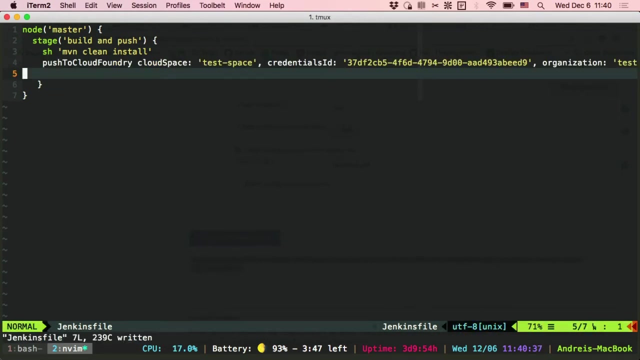 application to the Cloud Foundry. so here I need to specify the API which we will be use: credential, which already stored in the my Jenkins environment, some organization and some space, and generating a pipeline script. so so that's all. it's how our basic pipeline file can be, can be used, and you see that it's really easy to create using the this. 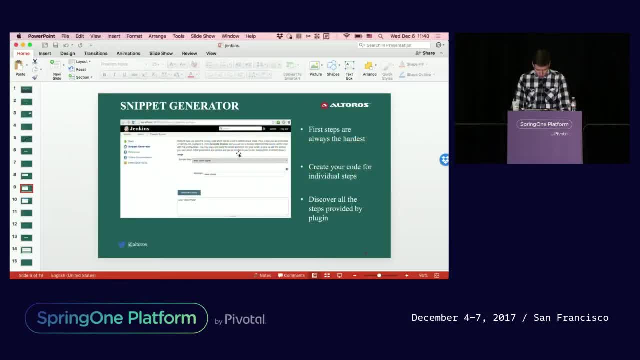 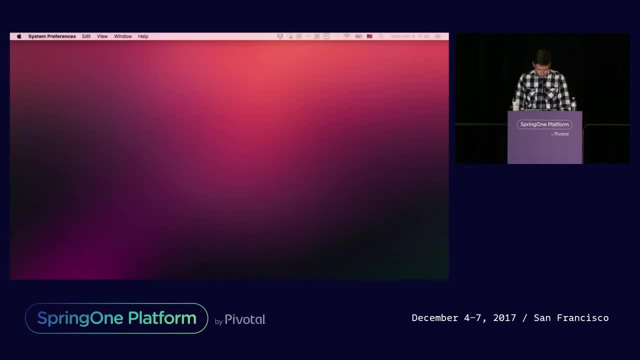 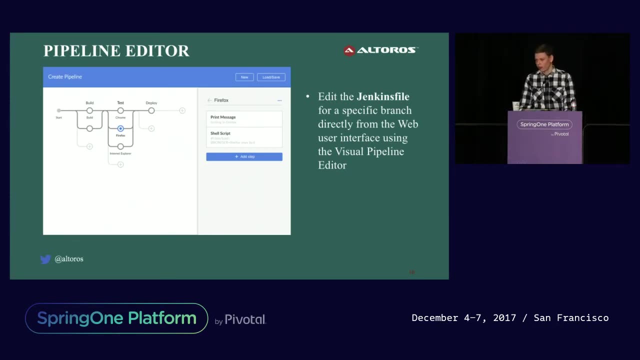 pipeline a snippet generator feature. so let's continue. it's my presentation. another one: how many of you are actually working with Jenkins? almost all, and how many are you using their blue ocean UI? okay, not many from the version, from the version Jenkins 2.0. Jenkins seclude out of the box. this is new UI. 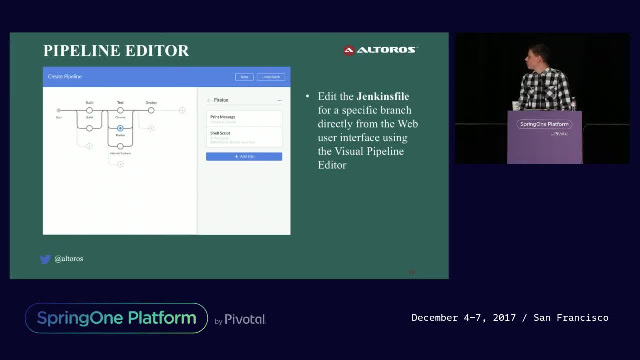 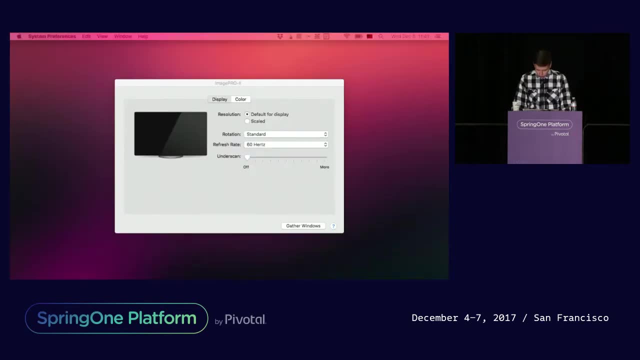 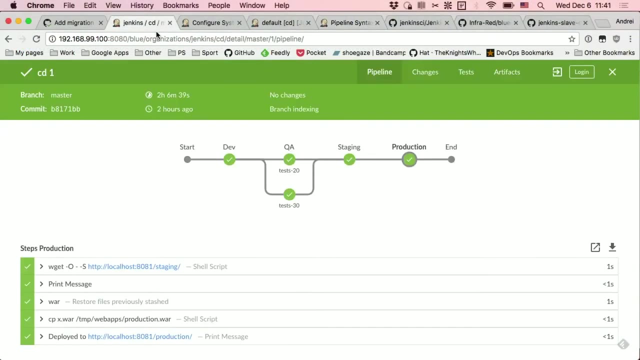 which is called blue ocean UI, and this UI includes some additional features which can be used to edit your pipeline files. so let me show how you can use the blue ocean pipeline editor with your Jenkins files. let's open. this is how the pipeline actually looks in the pipeline editor. so let's open my another job. 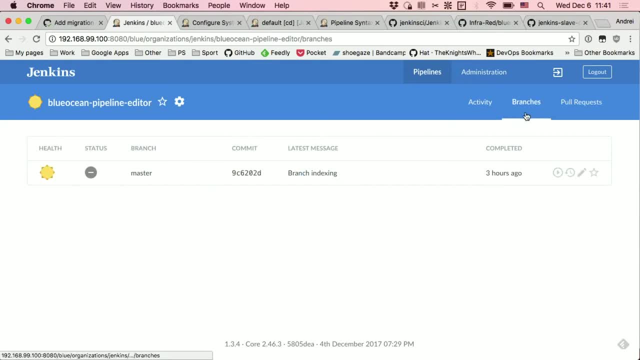 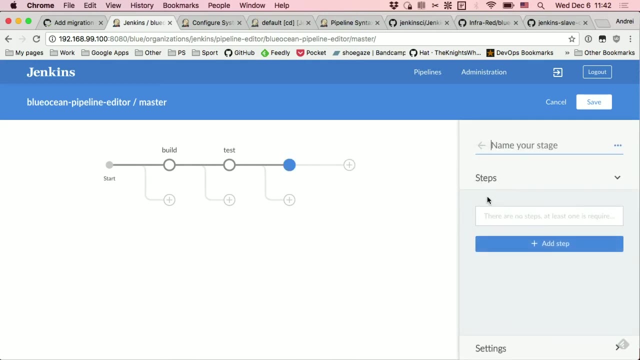 I have a job called Blue Ocean Pipeline Editor. open our branch and here we can easily add some steps to our pipeline file. As you see, I already have build test tasks, so let's add a new task which will push this application to the Cloud Foundry. 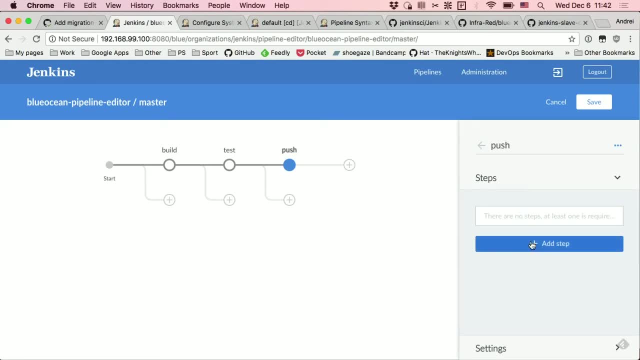 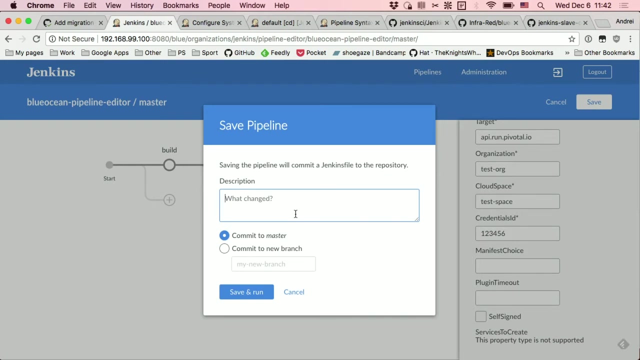 So we will call this stage push and add a new step which will push to Cloud Foundry and again some random credential ID and click save. And actually when we click save, Jenkins will automatically commit these changes and push these changes to our Git repo which we are using with this pipeline file. 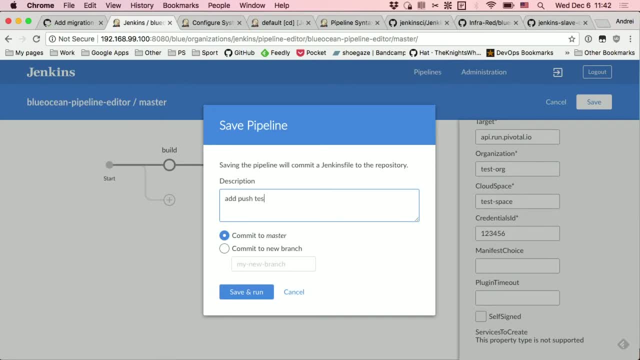 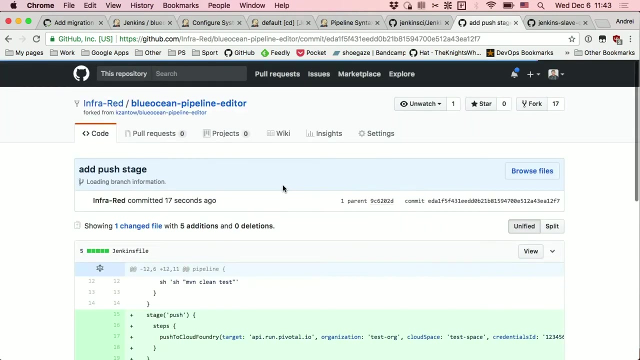 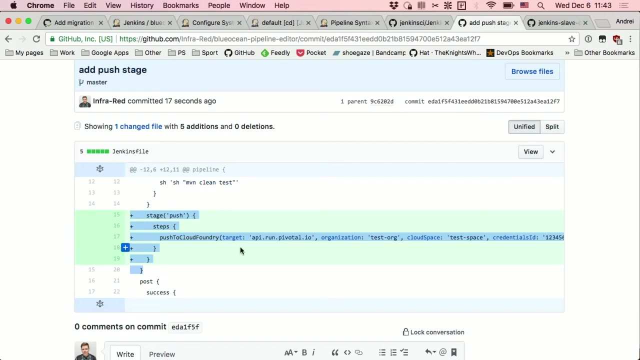 So let's check at push stage. Let's wait for some time to save the changes. Now we can change my repo And, as you see, the old changes were committed to my GitHub repo, So you can choose. would you like to change your Jenkins file from your favorite editor? 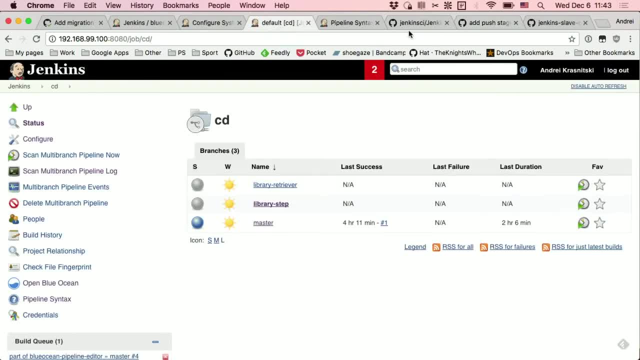 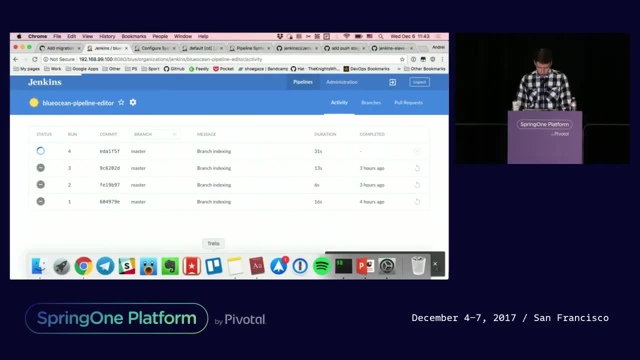 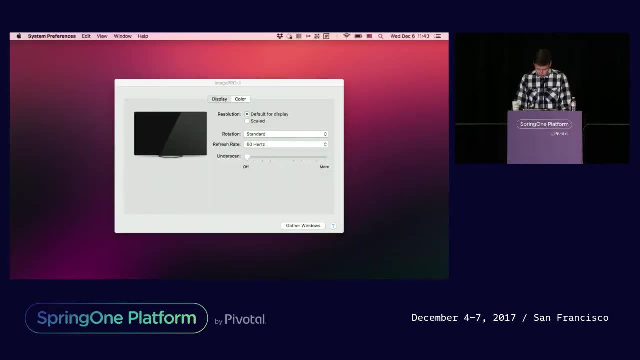 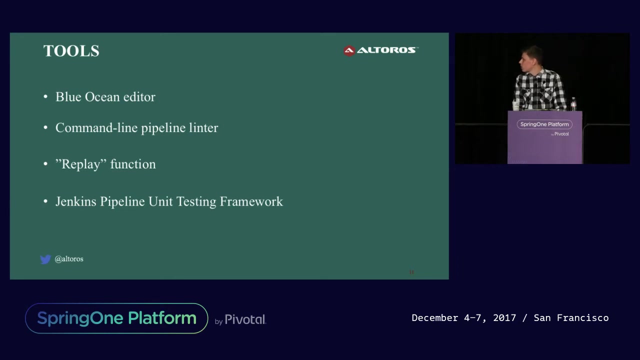 or you can just use this. You can use the Blue Ocean Pipeline Editor at some additional stages in this and Jenkins will automatically commit all this for you. So let's back to presentation. Jenkins also offers some other tools which can be useful when you're trying to improve. 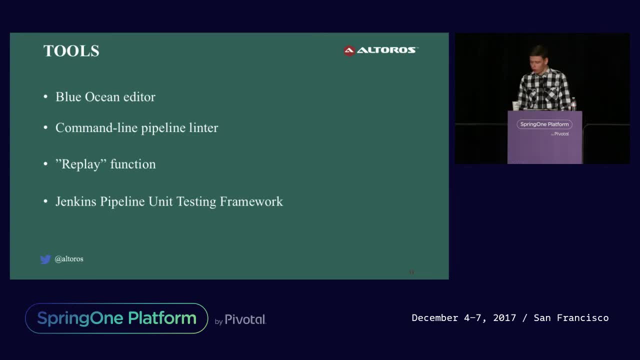 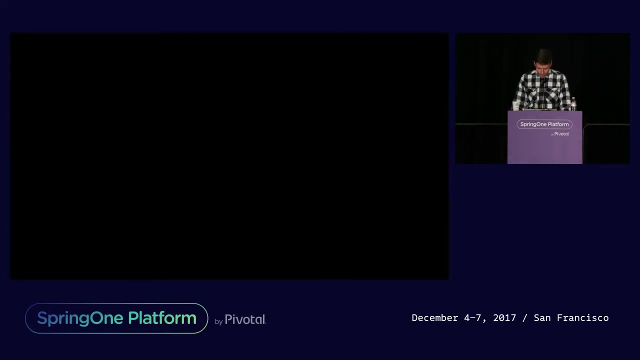 or debug your pipeline code: Blue Ocean Editor, One of them. I already mentioned about that. Then another tool called Command Line Pipeline Linter. It allows you to check and validate the pipeline code before actually applying these changes to Jenkins server, So we can use our file that we created before. 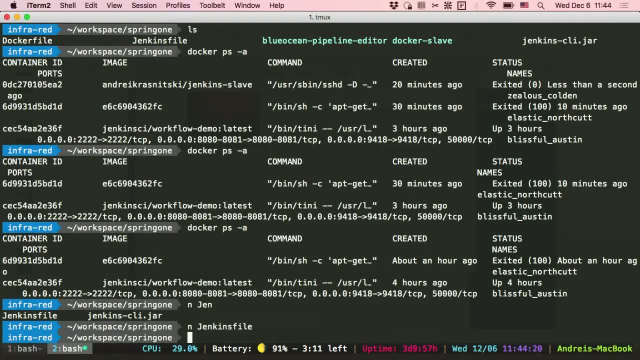 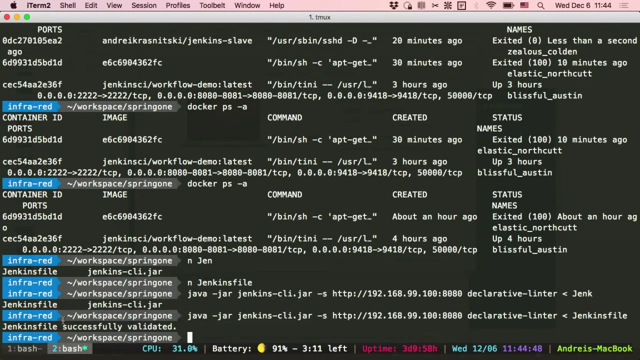 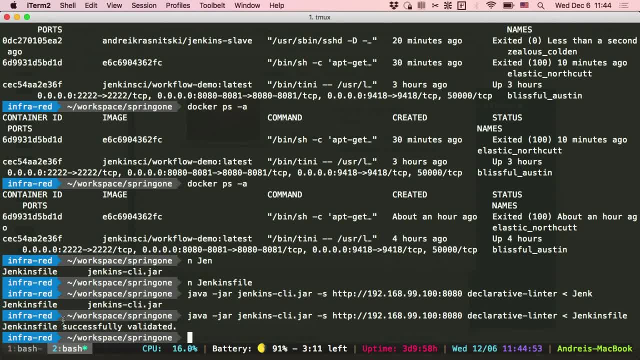 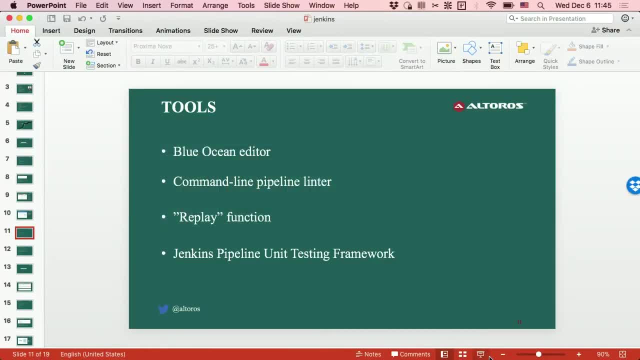 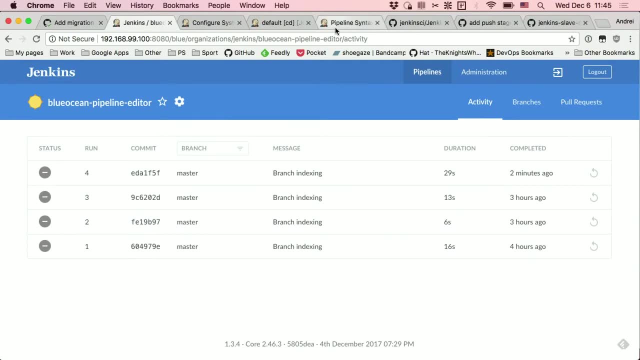 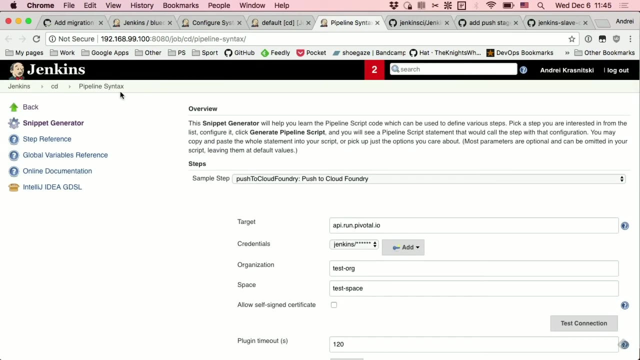 So you can be sure that syntax of your Jenkins file is correct and you can apply these changes to Jenkins server. So the next is Jenkins replay function. This function actually allows you to rerun your build if some of the steps were failed. For example, I can open this: 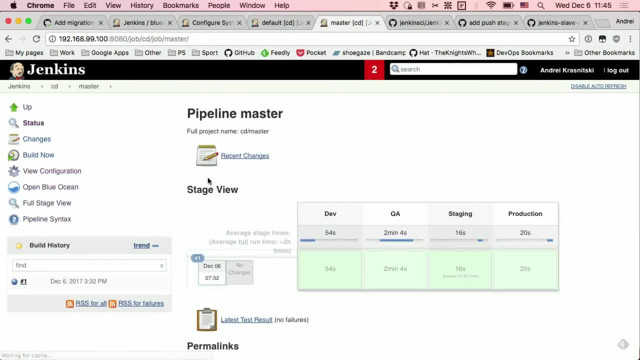 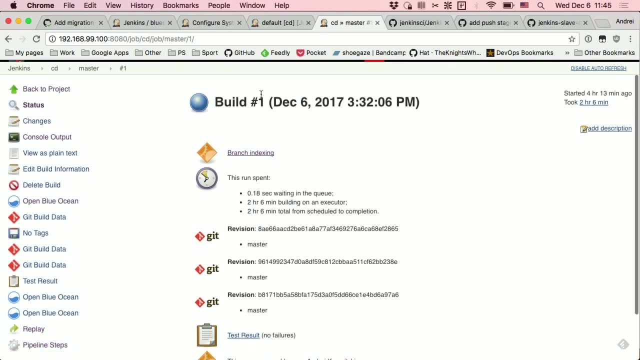 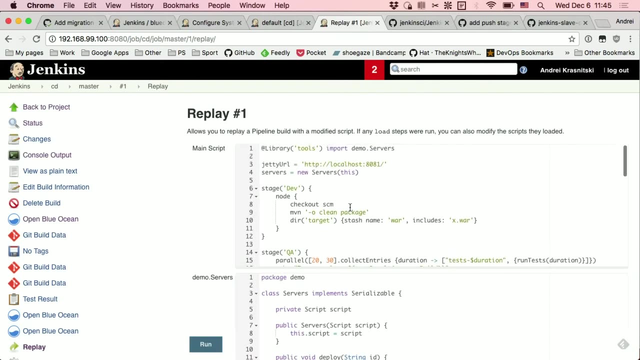 Okay, Open my job. I need to open some build. Let's assume that this build was not successful. but this build were failed And now you can click replay, change something in the pipeline script and just check before committing these changes to Git that your pipeline file will work with the new changes. 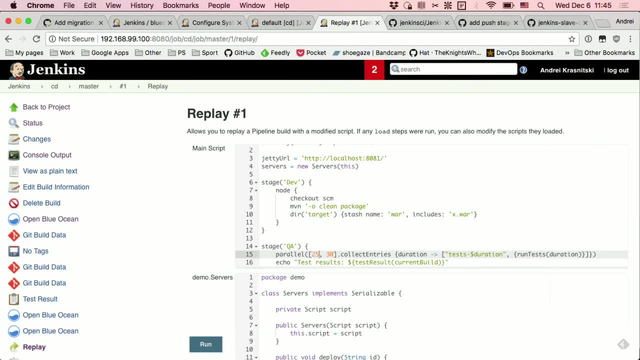 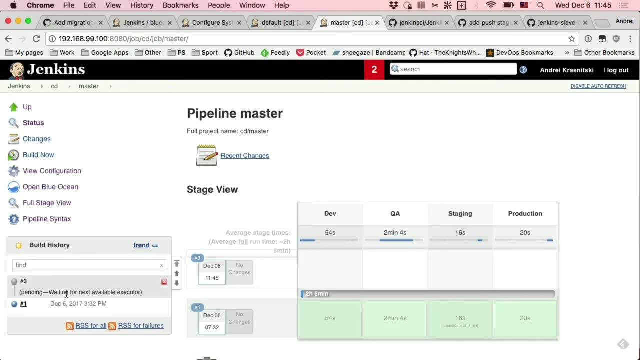 So let's check. Okay, Thank you. That's just a久 of my own experience. Just give me some time. Do we need to�KC TX and lol This duration file? You can click run and you will see this feature start running on the NSNow Jenkins. 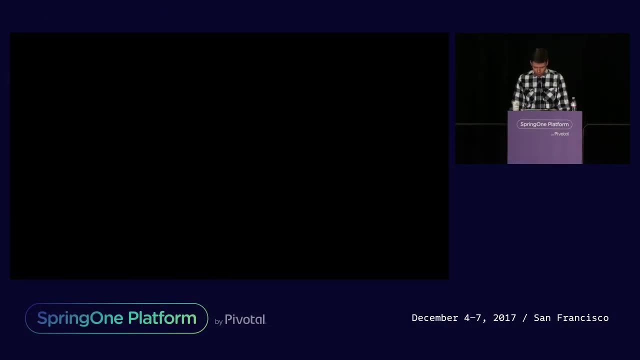 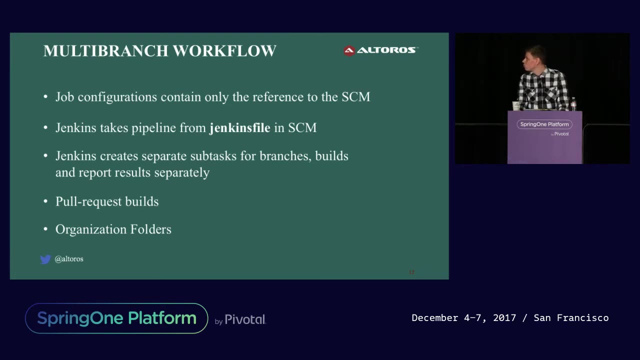 Workshop. Let's continue. Okay, So sometimes you need to work with the different in your single repository. Okay, For sure, you can just use the different. you can configure two jobs: point this to the single and select the different branches. 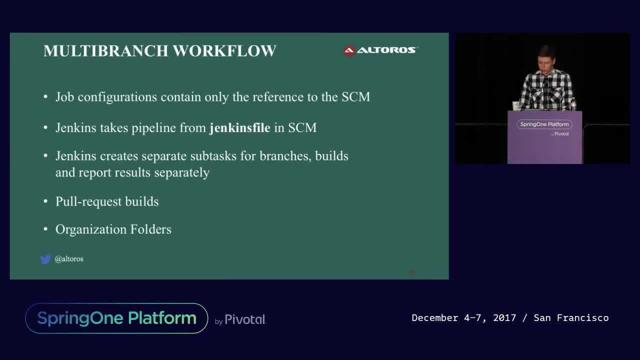 But in the recent versions Jenkins already offered the solution called the multi-branch workflow. It will automatically take the pipeline files from the old branches which are available in the repo and create the separate task for each of the branches. So you don't need to configure each of the branches separately in the Jenkins environment. 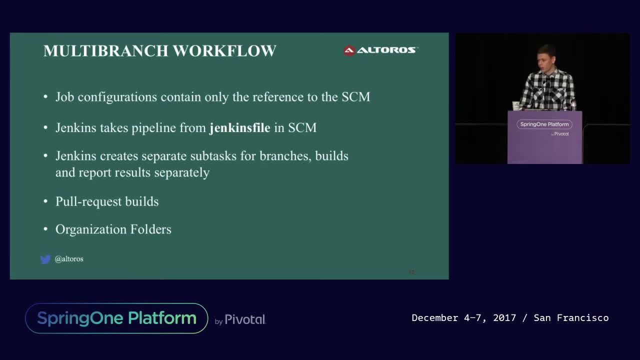 Also, if we can like use the different branches, why we can't use the whole? for example, GitHub account or GitHub organization, if we are all working on the same Jenkins server and we are included in the same GitHub organization? So for this purpose, Jenkins include the organization folder. 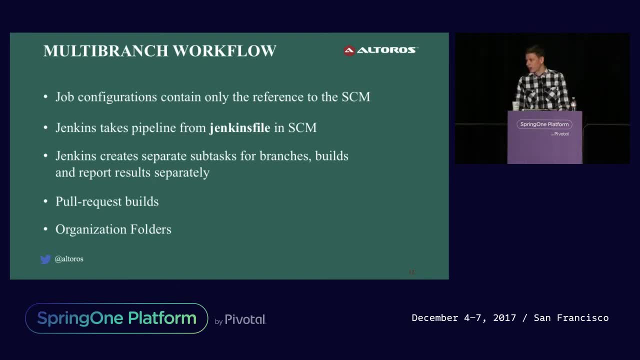 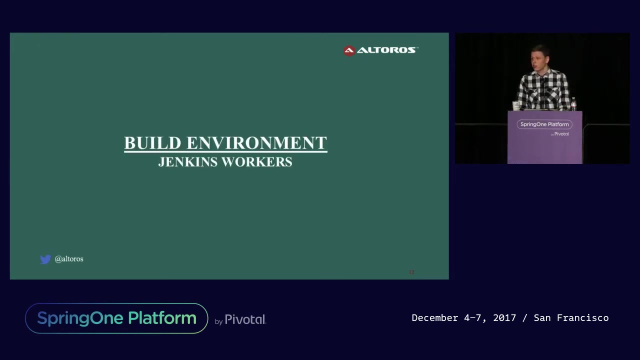 You can, Okay. So with the help of this feature you can just scan all the repositories available on the organization in the GitHub And if pipeline file is available in your repo, it will be automatically added to the Jenkins server and all tasks were created in the Jenkins server. 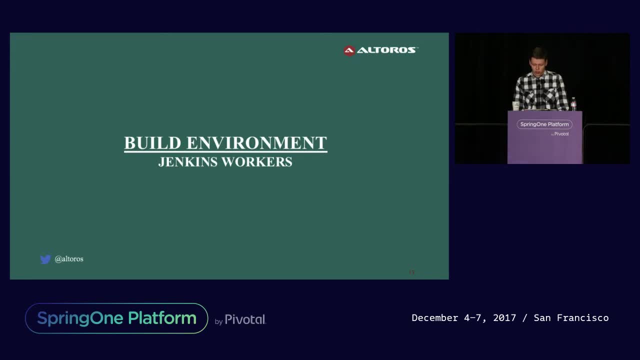 Another problem which we have faced when we was creating like our Jenkins tile for Pivotal Cloud Foundry, was the ability to provision Jenkins slaves which run in the builds with some dependencies which will be maybe required during the build process, And since we are trying to build like unified solution, we can just create the new tile. 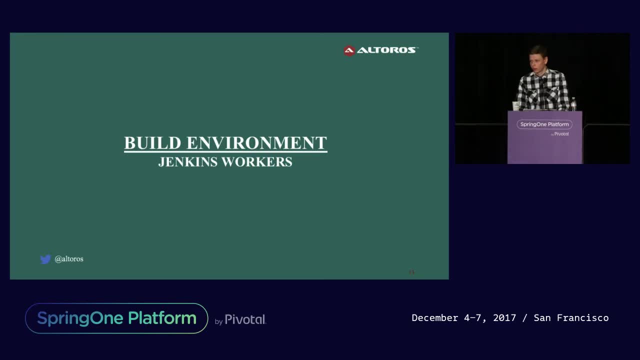 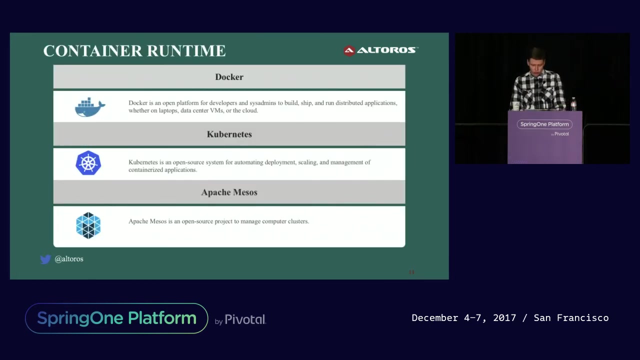 file for each of our customers with the different set of tools. We are trying to use the single tile which everyone can download from the Pivotal network. So most obvious solution for this will be to use the containers which will run our builds and sites. 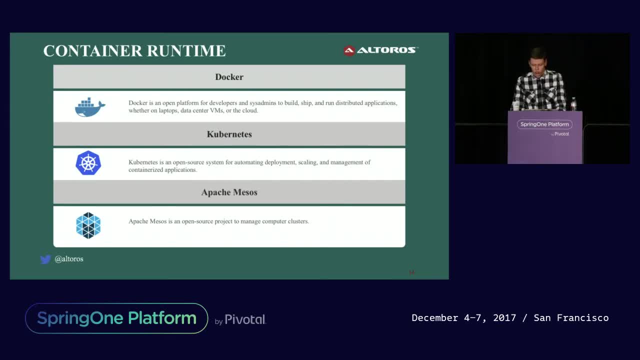 So most popular solution to use containers with the Jenkins is now the following. So most obvious is Docker, which we are currently using. We also consider to use the Kubernetes and Apache Mises, but these two solutions are really complicated And our task from maintaining the Jenkins server will become to another and more complex. 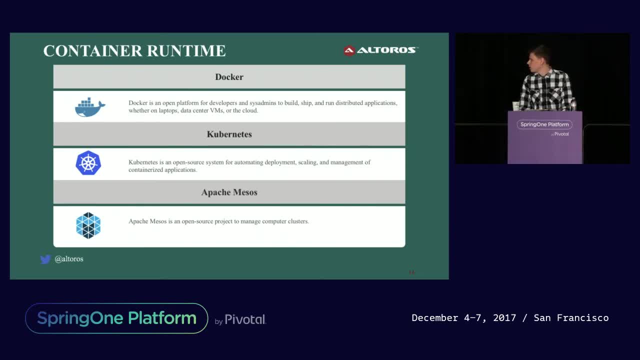 task like maintaining the Kubernetes server or Apache Mises cluster. But I'm really excited about the announcement of the PKS for the Pivotal Cloud Foundry. So in the near future we are planning to delete our Docker cluster, which we are currently 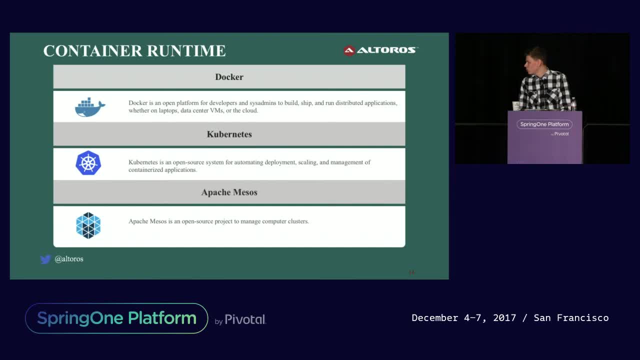 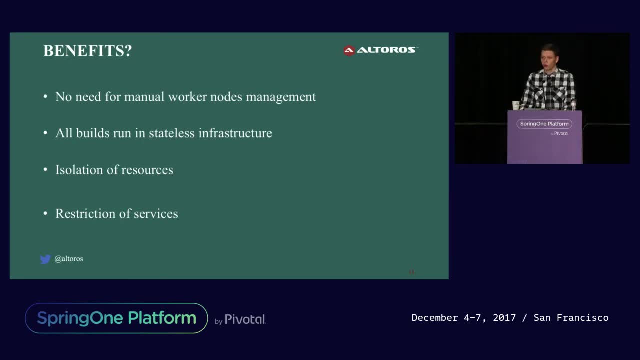 installing with the Jenkins PCF tile and we'll try to use the Shared solution which comes with the Pivotal Cloud Foundry itself. So what the problem? our containers help to solve us. As I said before, if you need to have some tool to be available during the build process, 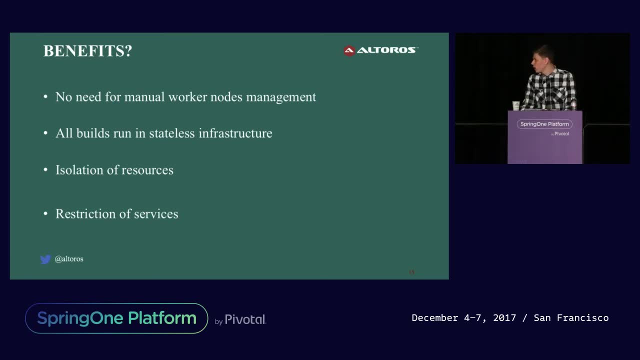 you just need to modify your Docker file at the couple of lines, which will install your favorite Ruby version, Python version, Go version, And that's it. So I think most of you already know how Docker files works, and this is not a complex task. 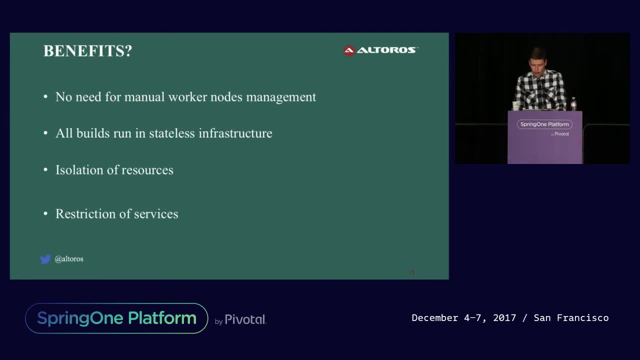 for you And another benefit- and actually this is the most important point- that each build will create his own container for build and each time you will have like fresh builds. So you may be almost 100 percent sure that all of your builds will be reproducible in. 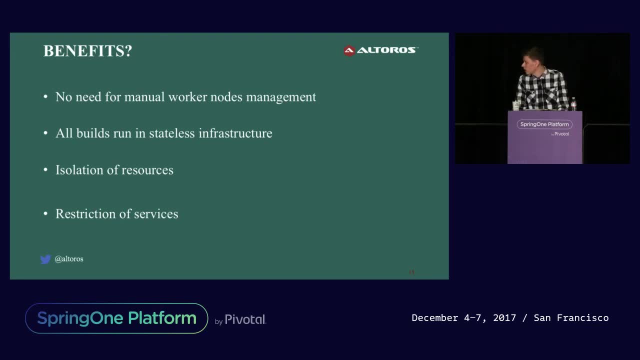 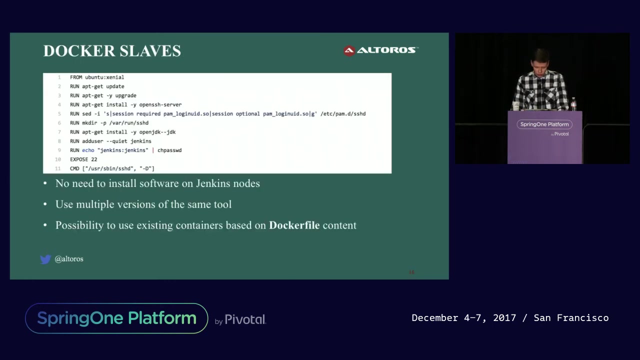 any environment Containers also provides us the isolation of resources. You can specify in Jenkins configuration that you want to allocate, like specific amount of memory or specific amount of the CPU, to our container and, configuring this way, our Docker clouds. So here example: how basic Docker slave, Docker file. 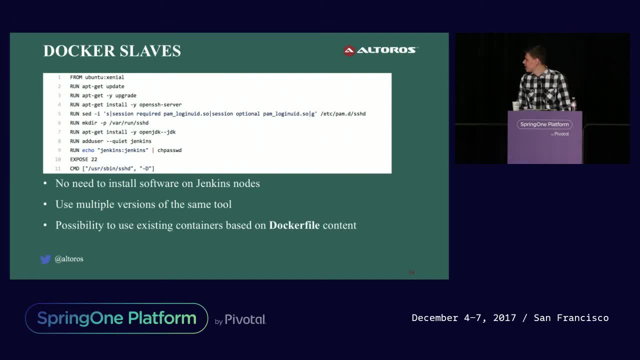 Do you see this? Yeah, Yeah, Yeah, Yeah, Yeah, Yeah. This slide shows how the basic Docker file to use as a Jenkins Docker slave we can use. As you see, it's neat- just to install the open SSH server, configure the Jenkins user. 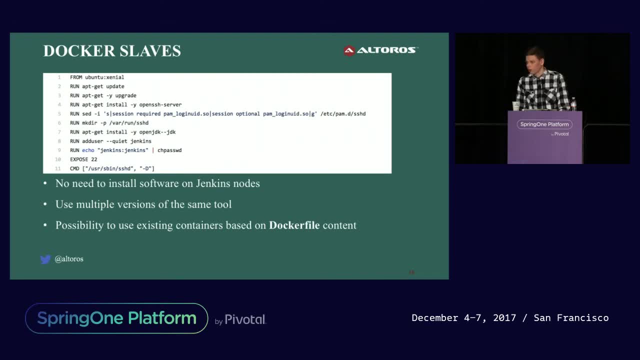 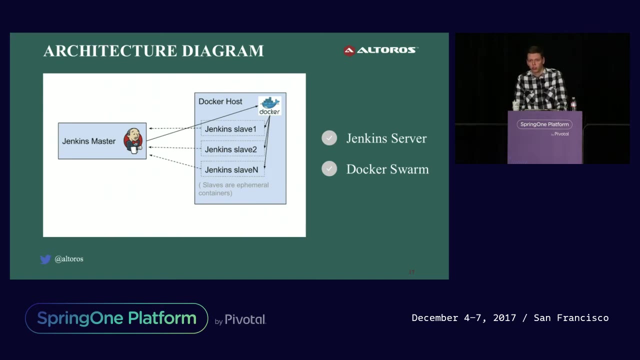 authorization using the SSH and that's all All other steps. it depends on you. You can add additional steps to install some stuff which you will require during the build process, and so on. This is current architecture of our Jenkins for PCF solution. 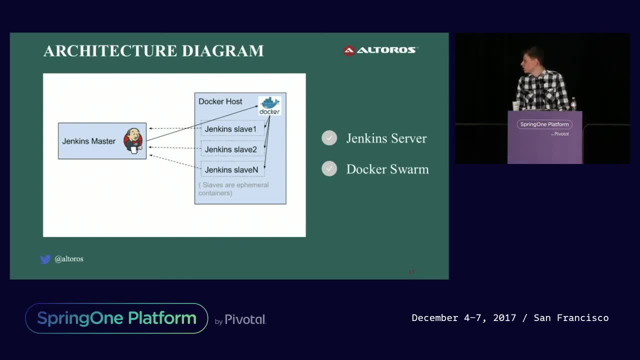 Basically, we installed the one Jenkins master and the Docker host single host or Docker swarms cluster, if you need to like many hosts which can run the Docker builds. And currently the problem which we are trying to solve is the high availability of the Jenkins. 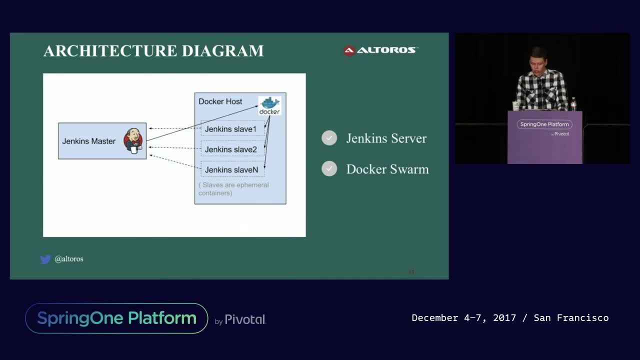 master, Which are already included in the Jenkins enterprise solution. but there is no typical solution for the open source version And, for example, we can use the shared file system. but this is configuration a bit tricky and we are trying to solve it somehow. 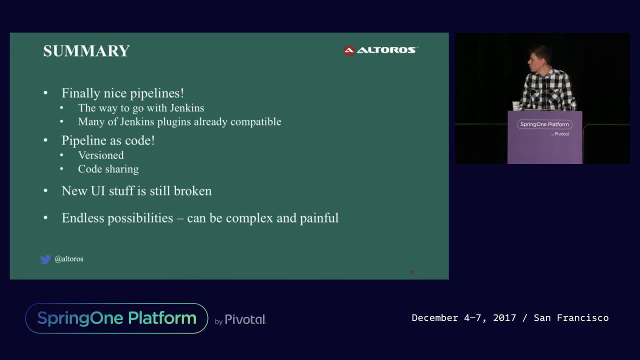 So this is like a short summary for my talk. Finally, Jenkins, include pipeline so you can build like complex logic for your software, For your CI CD process. I also want to mention that not all the configuration is available currently in the UI, So if you plan to use, be aware of it. 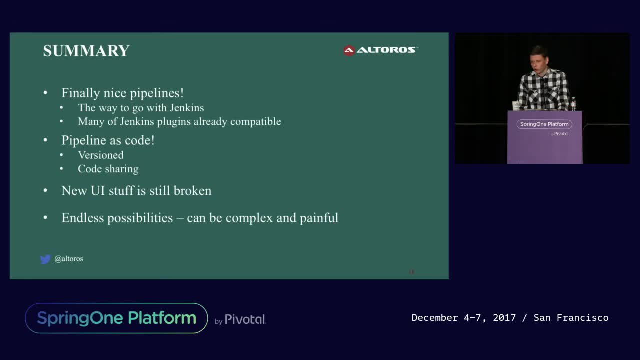 And I again want to say that you should always start your project by implementing the CI CD process. It will be much easier to maintain your pipeline code when you start it and not when you have like a thousand. And it will be much easier to maintain your pipeline code when you start it and not when you have like a thousand code lines in your repository. So this is it, Thank you.